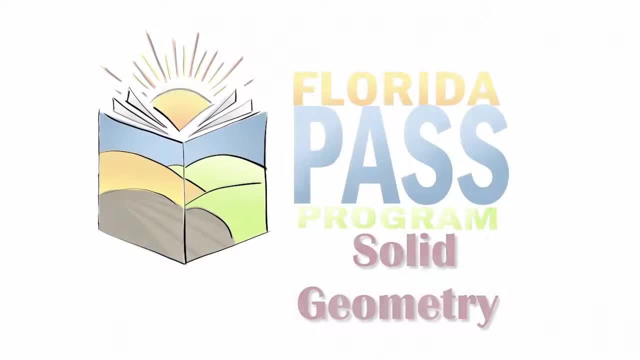 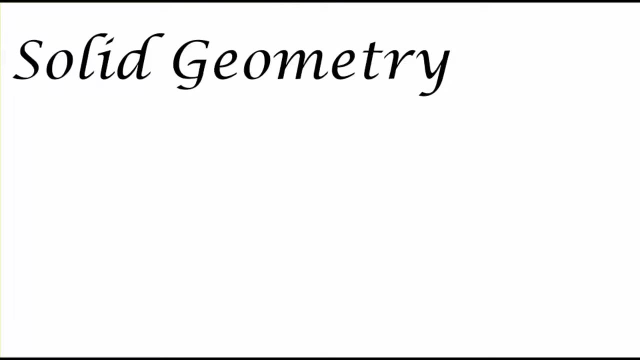 Welcome to the lesson on solid geometry. In this lesson we will take a look at 3D figures and how we go about classifying and identifying those figures on their characteristics. Solid geometry is a part of mathematics that deals with three dimensions. Three-dimensional figures are called polyhedrons, which is essentially a three-dimensional shape. 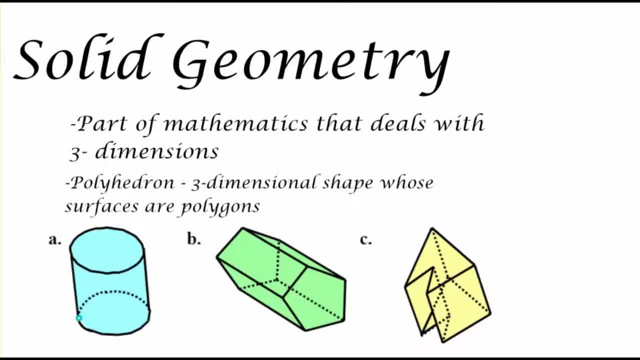 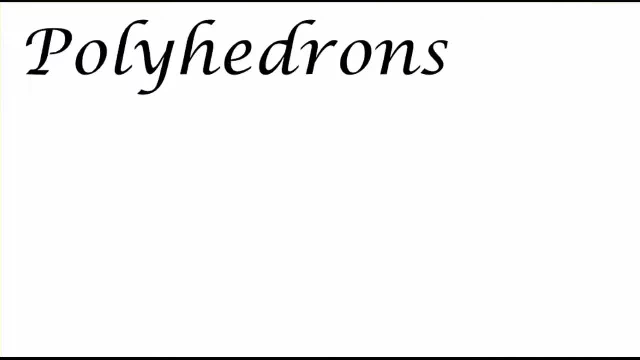 whose surfaces are polygons. Now, looking at these three shapes, one of them being very recognizable, we would know that the second two are polyhedrons and the first is not, for reasons that we'll discuss in a little bit Now. polyhedrons have a variety of characteristics that can often be counted and help us identify and describe. 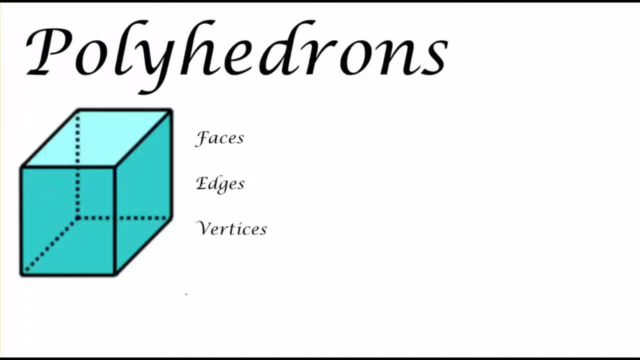 which ones we're talking about. So when I think about the faces of my polyhedron, I'm thinking about the flat sides, In this case of a cube. we know that our faces are squares. So as I count the faces, I know that this square polyhedron will have six faces. 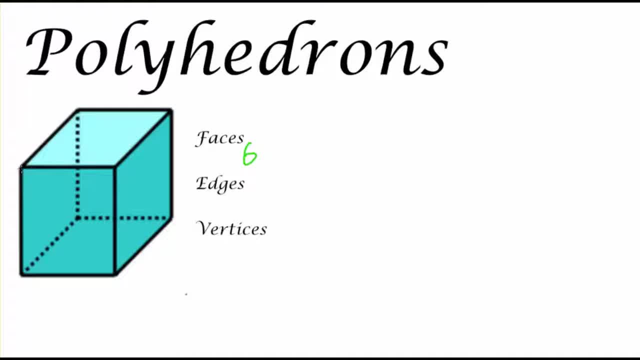 You can look at the four edges on either side and the four edges connecting those two sides, giving me a grand total of 12 edges. Vertices: I have four on the bottom, four on the top and I have eight vertices with this polyhedron. 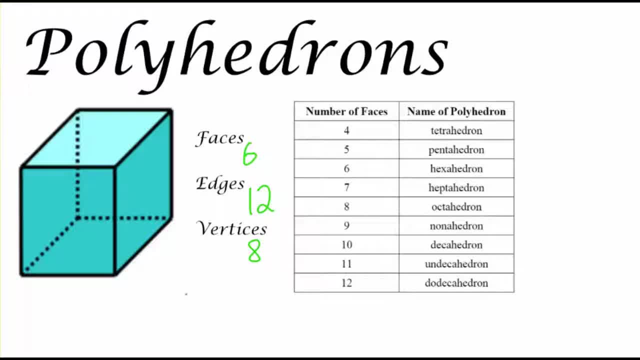 Classification-wise, it's important to think about the amount of faces and how they'll give each polyhedron a name. Four faces will give me tetrahedron, all the way down, following the pattern of the prefixes, to 12, where I would have dodecahedron. 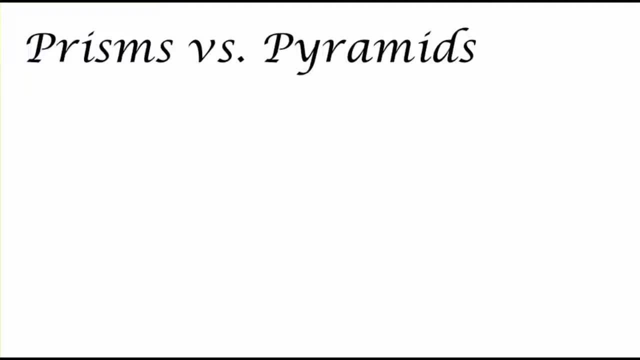 extending toward infinity. Now polyhedron can come into two basic categories: prisms and pyramids. A prism is defined by its two congruent bases and a connection of those bases, and the pyramid is defined by its one base and its lateral faces all. 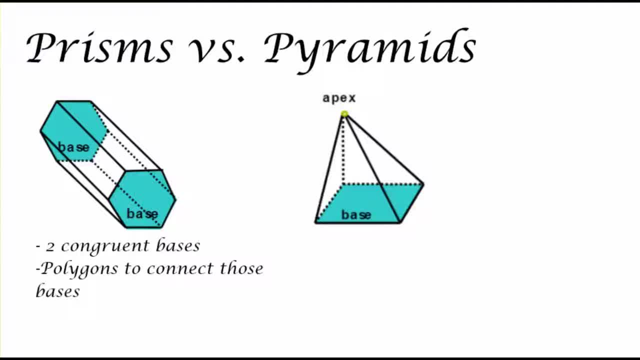 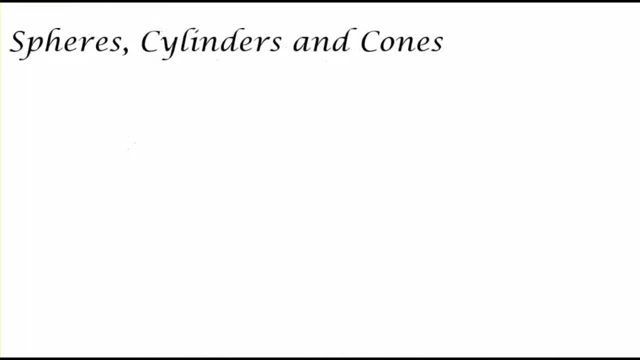 facing towards the apex, Again with the prism. those polygons are connected by the lateral areas and with a pyramid. our lateral areas, which are usually triangles, all connect at a top apex. These will be very important characteristics to remember when it comes time to calculating surface area and volume.